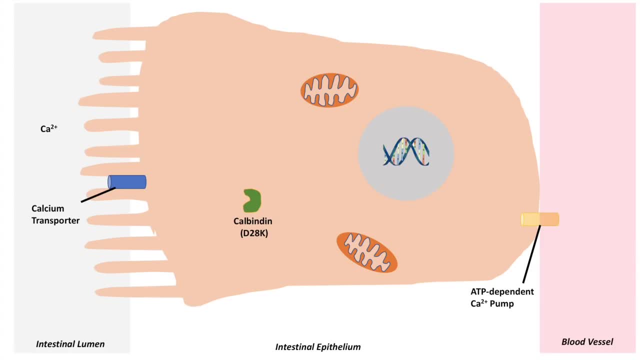 absorption and utilization. So why is that? Well, when we look at an enterocyte in the small intestine on the left, we can see the intestinal lumen. So say, you've absorbed or ingested some calcium in your diet. Well, the process, the basic process, 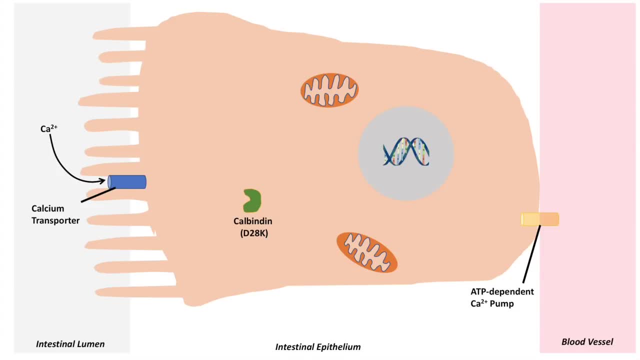 of calcium absorption goes like this: Calcium is brought into the enterocyte through a calcium transporter. It binds to a protein in the cytosol known as calbindin D. This allows the calcium to be transported through the enterocyte and to the opposite side of the enterocyte so that it can be. 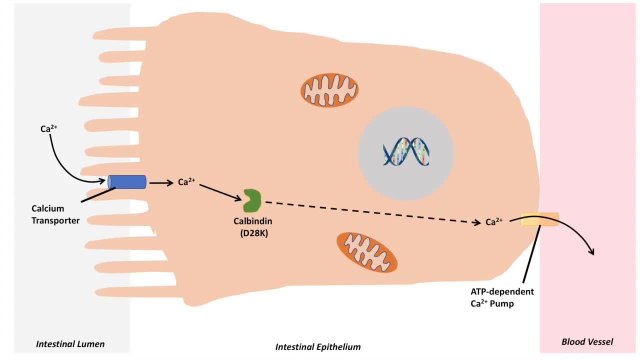 transported into the bloodstream via an ATP-dependent calcium pump. So why is calcitriol so important in this process? Well, when you have calcitriol, it enters the enterocyte and it'll actually bind to a protein known as vitamin D receptor or calcitriol receptor. Now this 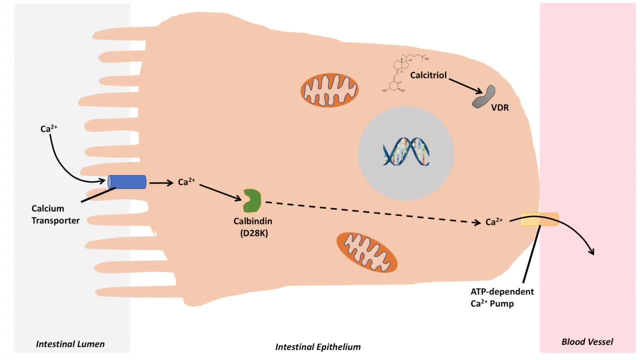 receptor is actually a transcription factor and it'll actually bind to something else known as retinoid X receptor, but that's not important in this process. So when it binds to vitamin D receptor, the calcitriol will enter the nucleus where it'll activate a. 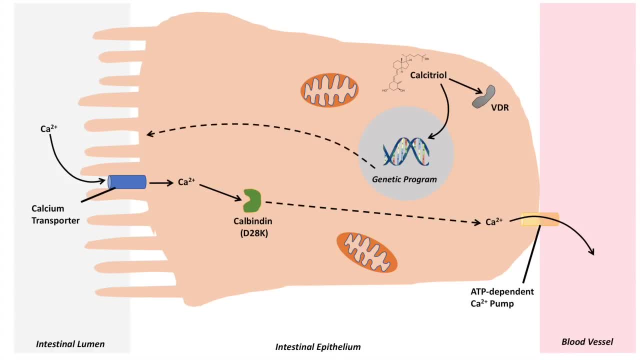 genetic program. So what does this genetic program do? Well, the genetic program will actually increase the expression, the transcription, translation and expression of calcium transporters, So that allows the enterocyte to uptake more calcium. It'll also actually increase the expression of 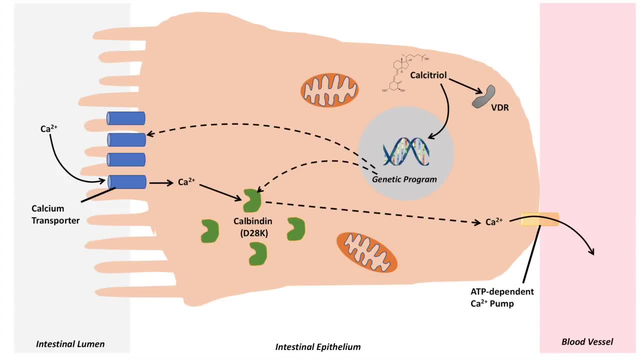 calbindin D, So it'll increase the amount of calbindin D within the cytosol. And, last but not least, it'll also increase the activity of the ATP-dependent calcium pumps to allow the enterocyte to pump out even more calcium into the bloodstream. So all of these processes will increase the uptake of. 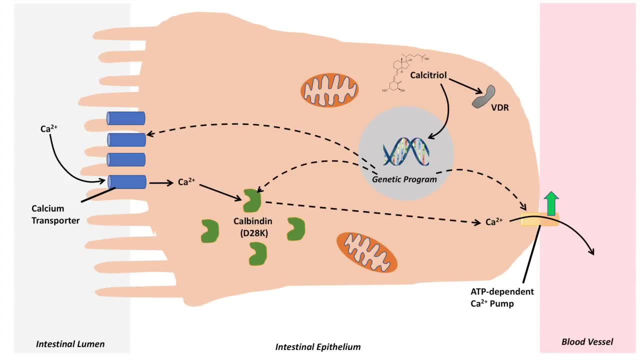 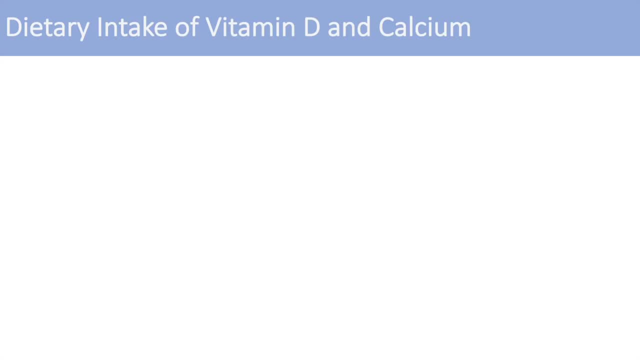 calcium into the enterocyte and allow more calcium to be uptaken or absorbed into the bloodstream. So what is the recommended dietary intake of vitamin D and calcium? Well, according to the National Institute of Health, the recommended dietary allowance for vitamin D in early life 0 to 12 months.